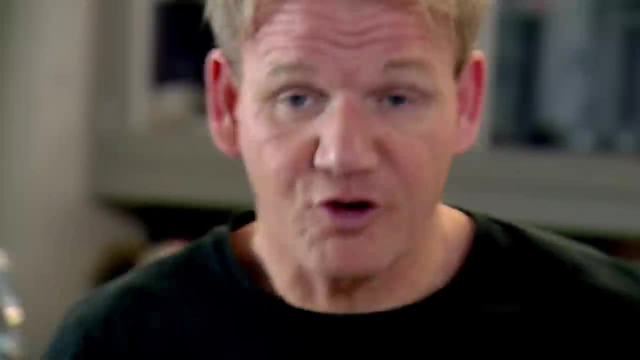 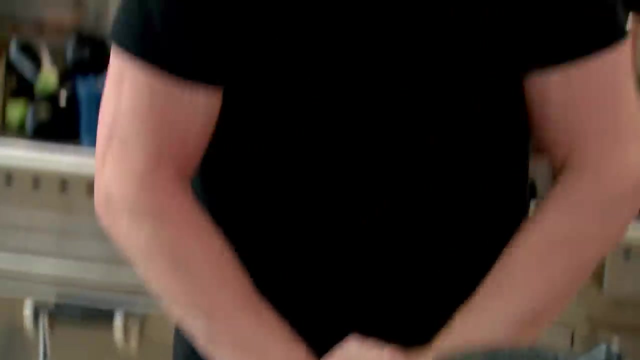 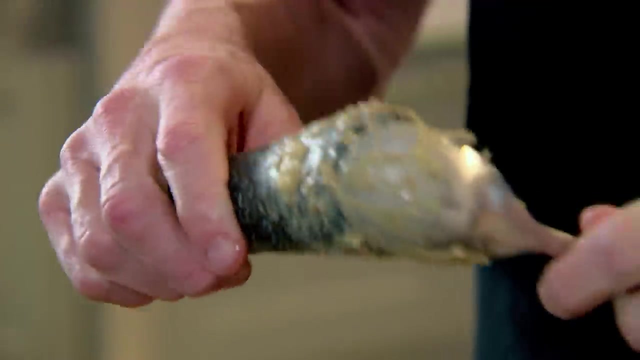 but in mine they're the base to the dressing. We're going to grind that into a paste And then get the garlic in there. Season well with black pepper- It doesn't need any salt in there because of the anchovies. Add a couple of tablespoons of red wine vinegar. 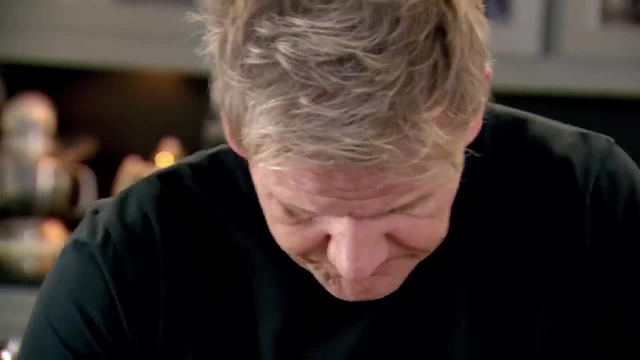 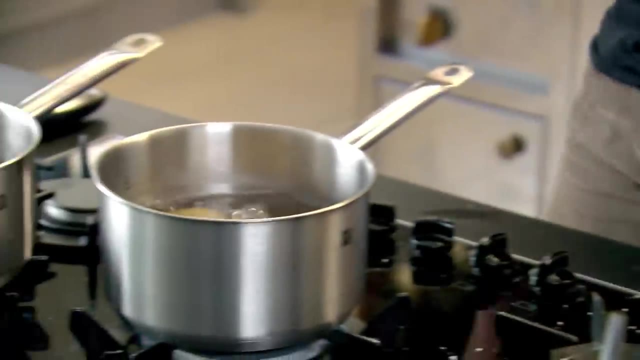 olive oil and lastly parsley to give the dressing freshness against those deep flavors. It's a thick, rich, substantial dressing. Dressing done Now for the salad: Boiled potatoes, green beans and eggs From a rolling ball. seven and a half to eight minutes. 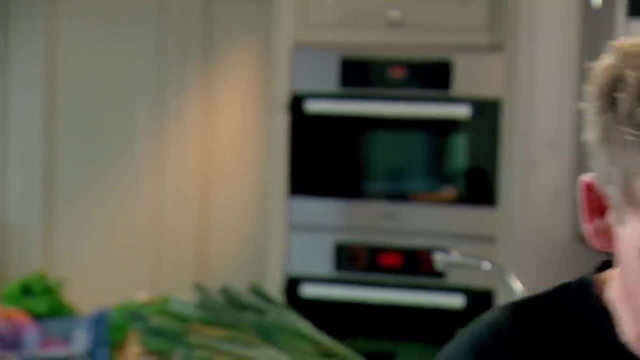 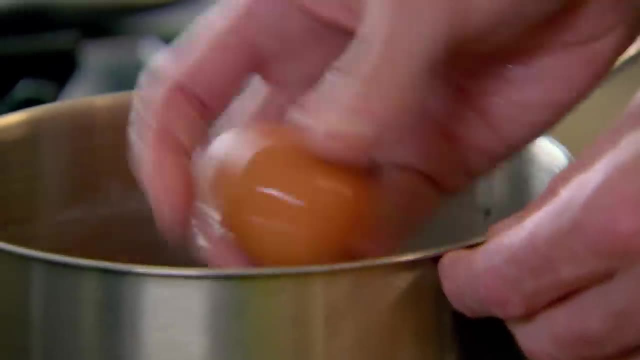 It should keep that nice yolky creamy texture in the center. Once the eggs are ready, put them into cold water to stop them cooking, and this is a great trick to peel them. It's so much easier peeling eggs when you use the water. 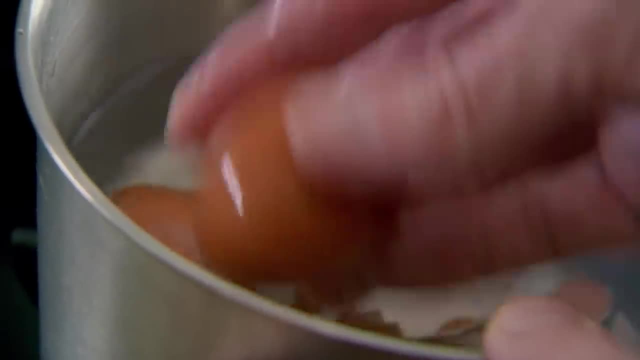 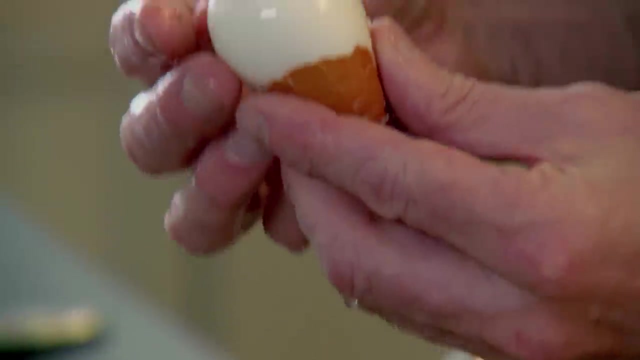 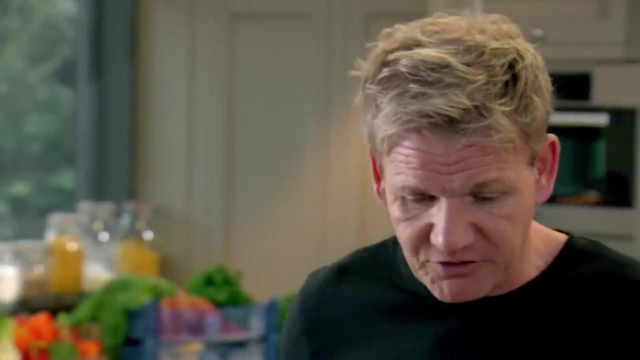 that they've been cooling down in, And the water will seep underneath all the shell, and so the whole shell just gets peeled off with one beautiful big layer. Now beans, Mmm, Nice and crunchy. Season the beans and potatoes whilst they're still warm. 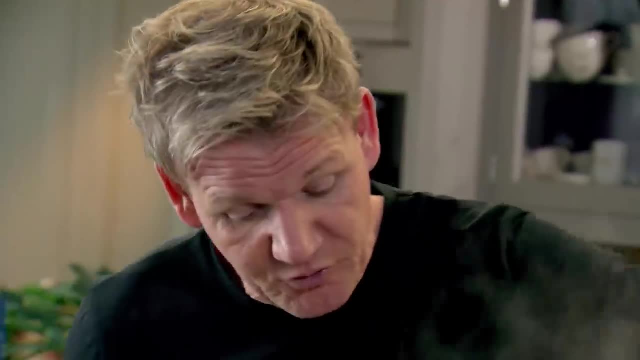 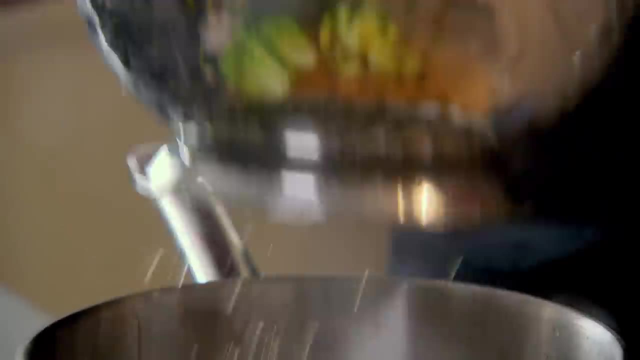 so they absorb more flavor. A little drizzle of olive oil, salt pepper and just let them sit there Whilst the potatoes and beans cool down. I'm doing a simple French toast, I'm doing a simple French open sandwich, which is called a tartine. 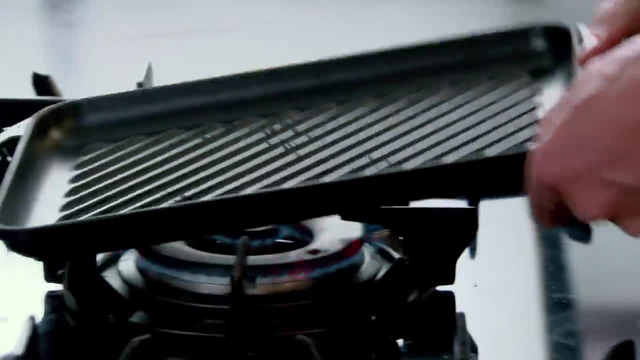 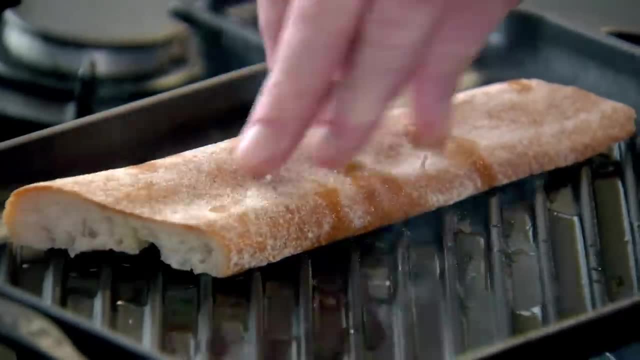 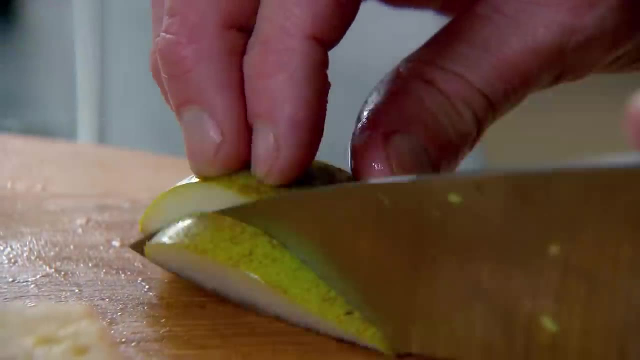 This is delicious. First I'm toasting baguette on the griddle. Lightly oil the griddle pan. Get your bread, Stick it on there. Take a pear: It goes brilliantly well with goat's cheese. Slice the pear into finger-width pieces. 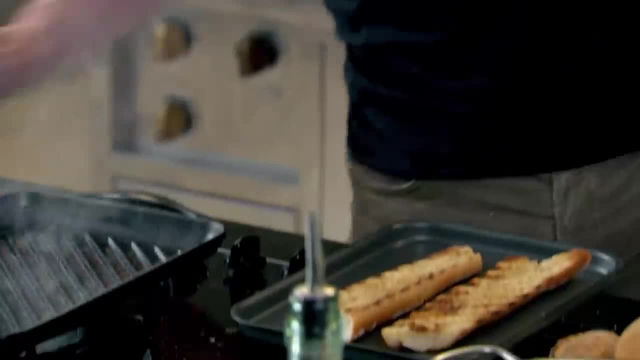 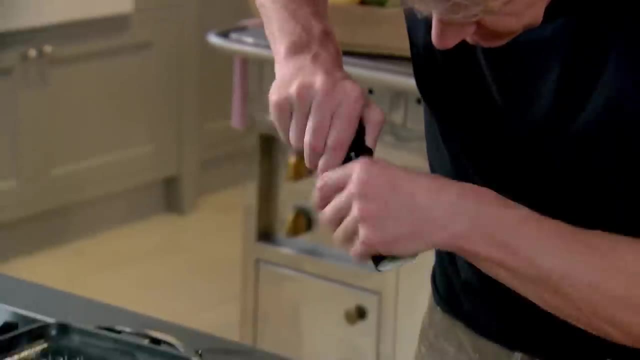 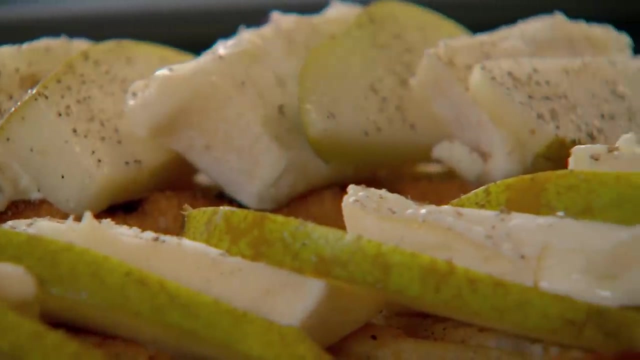 That's the color we're looking for, That dark crispy texture. Now for the goat's cheese. Give it a season. Doesn't need salt, cos a little fresh goat's cheese is already quite salty. Then a handful of crumbled walnuts. 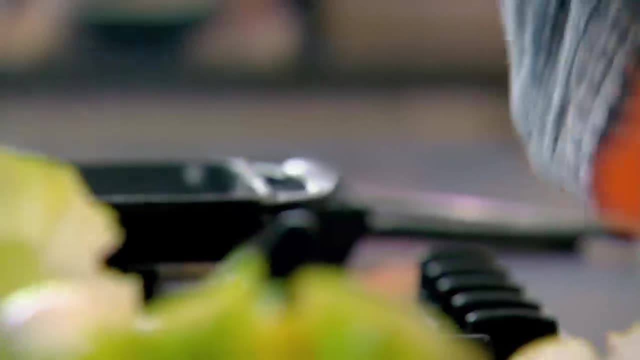 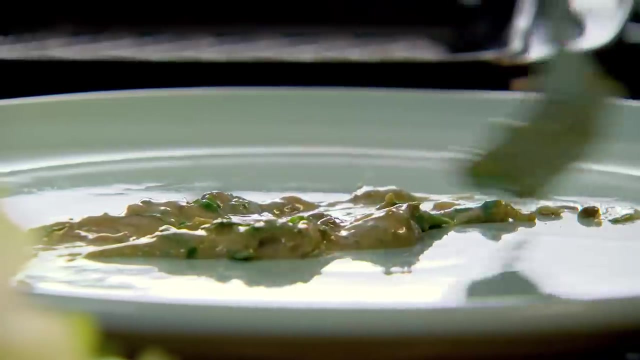 They go under the grill whilst I put the tuna niçoise together. My secret to assembling a great niçoise salad is to start in the middle of the plate and add ingredients layer by layer. There's one thing I'm always missing at the bottom of salads is dressing. 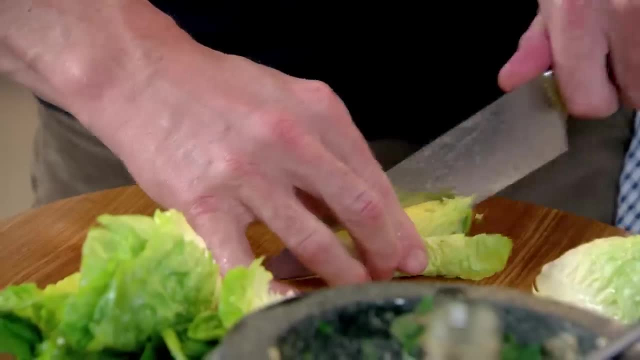 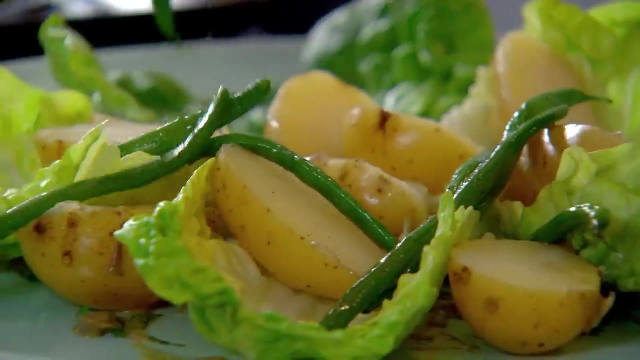 so I like to put it on the plate first. Baby Jim lettuce is great because it's robust and holds that heavy dressing. Then add firm waxy salad potatoes and green beans. I like them to have a bit of a crunch. Canned tuna can be fantastic. 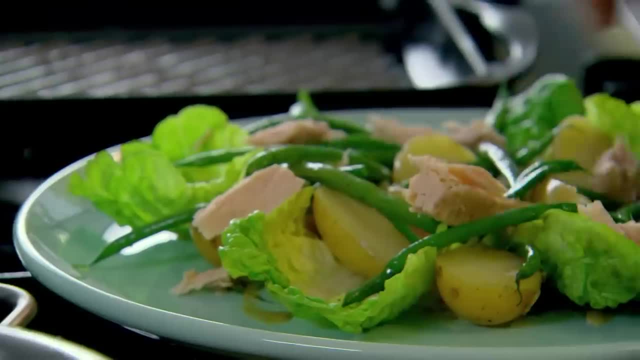 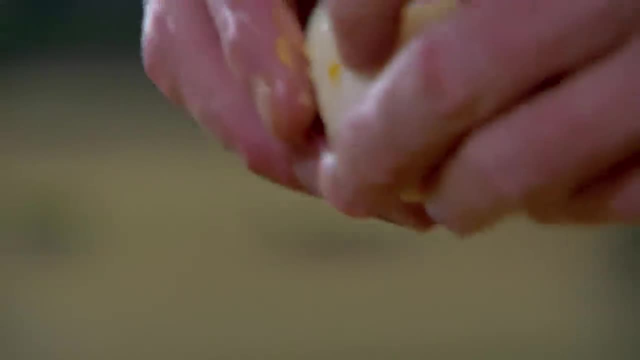 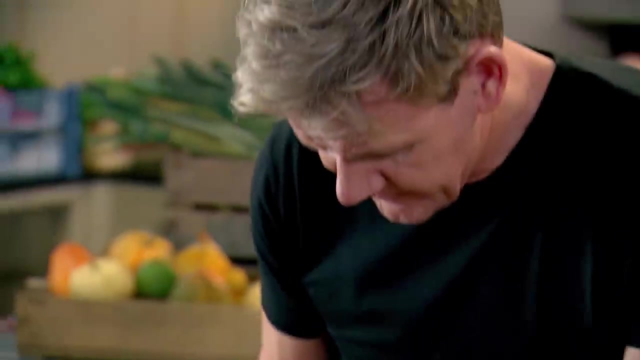 I'm using a good quality one in olive oil which has been drained. Next, baby plum tomatoes, which have a lovely, intense sweet flavor. And then my eggs, That nice, dark, rich yolk, Beautiful, The yolk's still creamy inside. 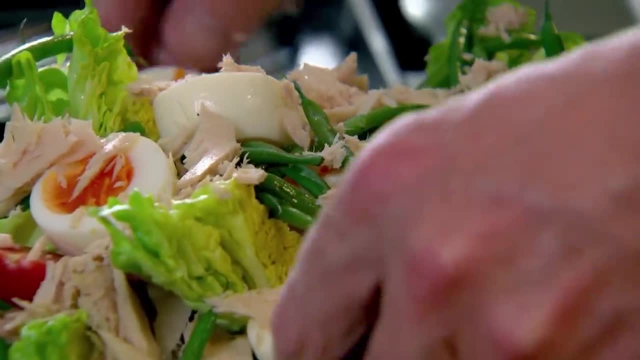 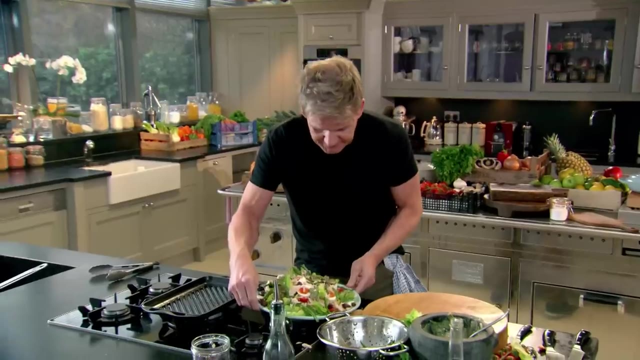 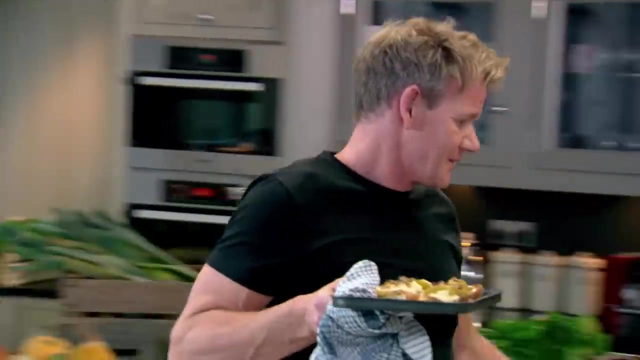 These are little olive niçoises. This will work just as well with other black olives. And then your dressing: Drizzle that round gently. Beautiful, That is a niçoise in heaven. Now tartine. Wow, Just the smell of those grilled walnuts. 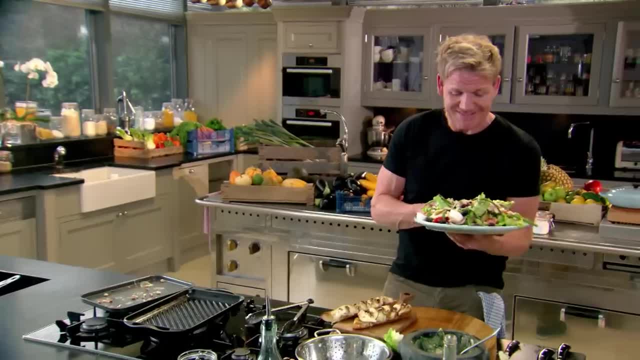 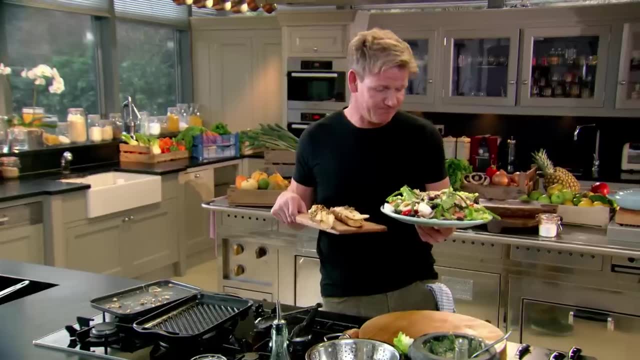 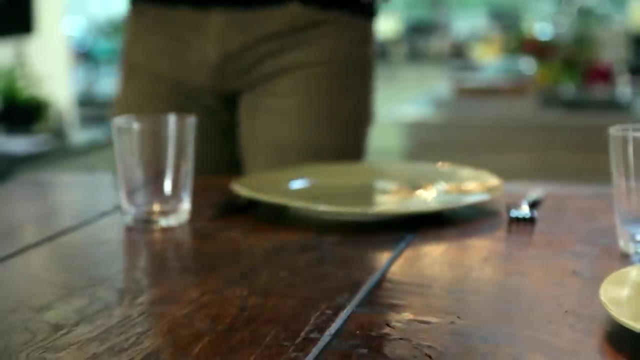 That is beautiful. A simple but very elegant tuna niçoise with a delicious goat's cheese sandwich. Wonderful, My vibrant and gutsy niçoise salad with that incredible anchovy and caper dressing, served with a pear and goat's cheese tartine. 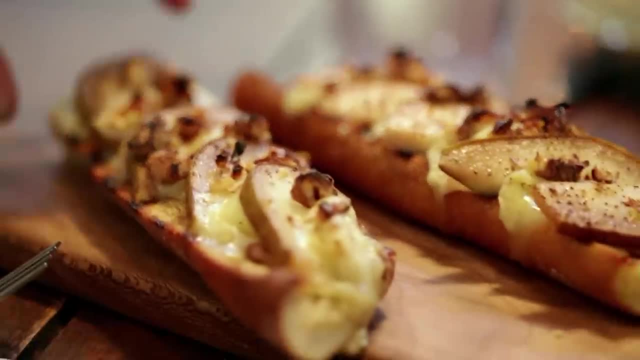 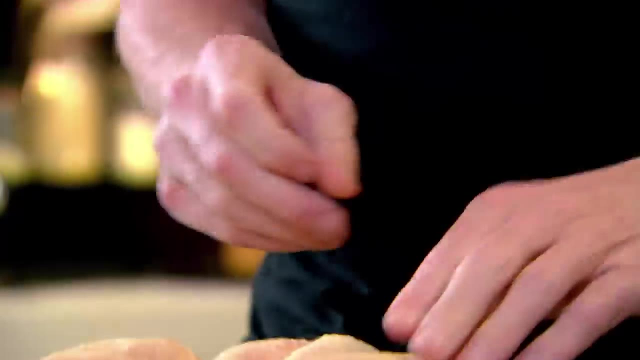 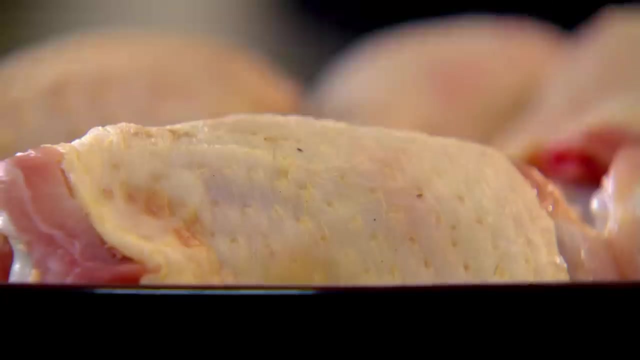 too good to let the French keep it all to themselves. Tilly, would you mind helping Daddy with the chicken fricassee please? We're gonna start off with browning all the chicken off nicely. Pan on, Get that nice and hot. 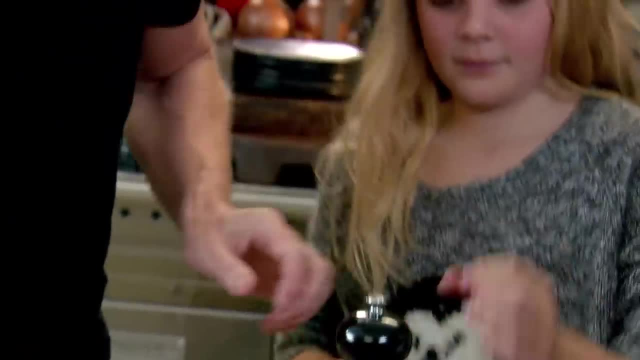 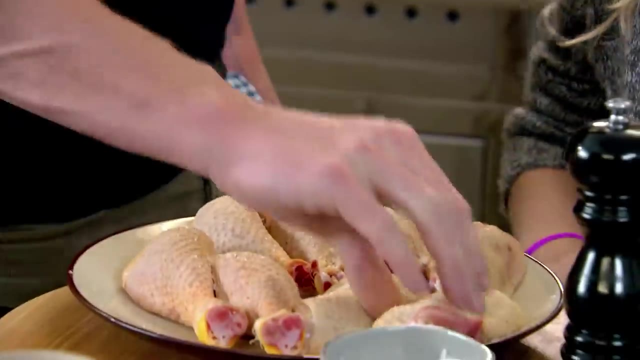 What I want you to do for me first is to season the chicken with salt and pepper, please Thank you. So that's on one side. Then we turn the chicken over, So we season it on this side, So we season it on the other side. 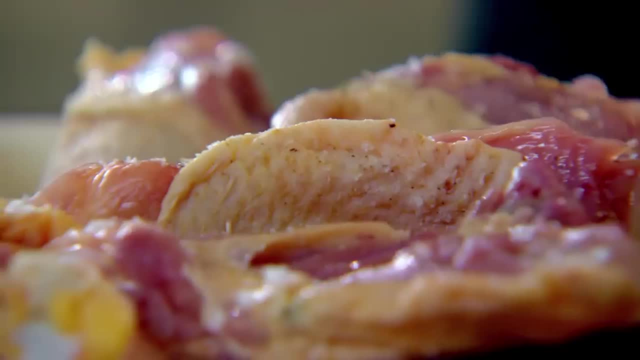 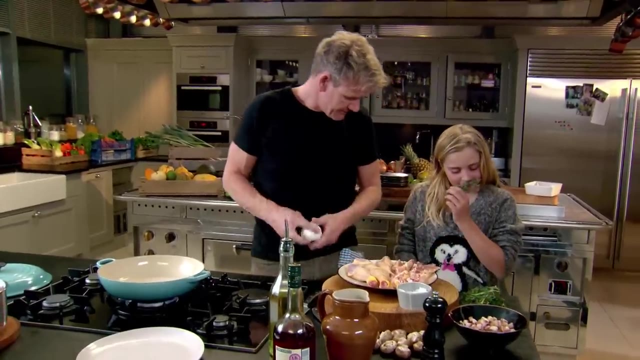 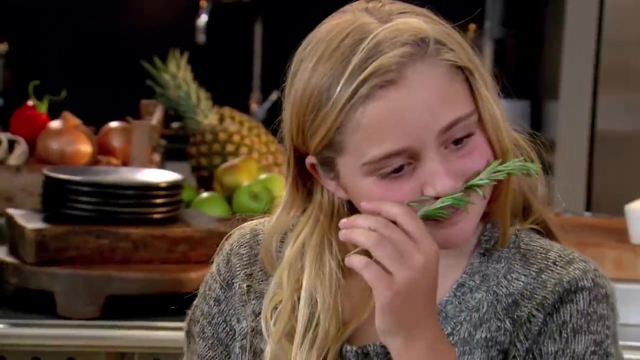 Salt, Good girl, And pepper, Nice. Now, this is almost like a chicken stew. OK, What's that there? Thyme, Thyme, Good girl. What's that one there? That one's rosemary, That's right. 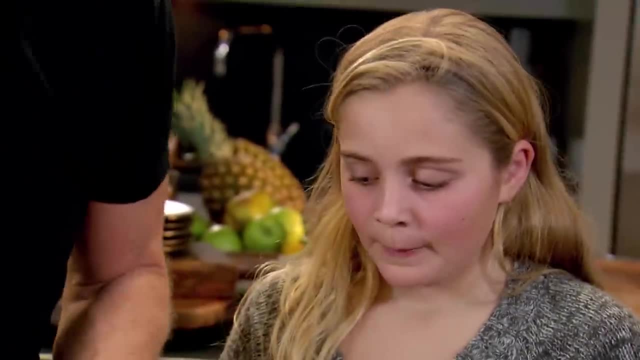 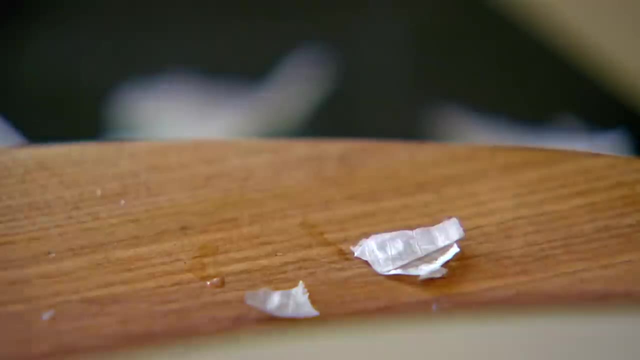 Rosemary, And because this is quite a rustic French dish, we don't need to chop everything. So we get the garlic And you just bash it like that. Now smell Mmm, Ooh Right, So that's nice and hot. 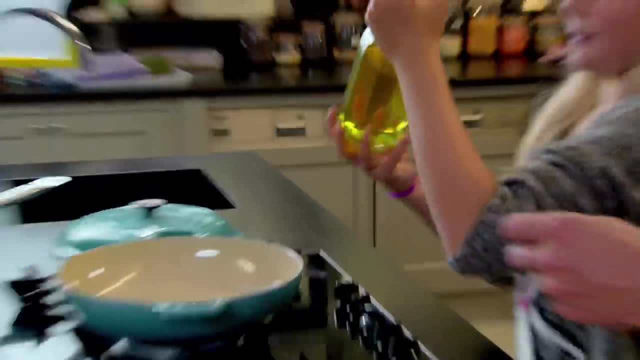 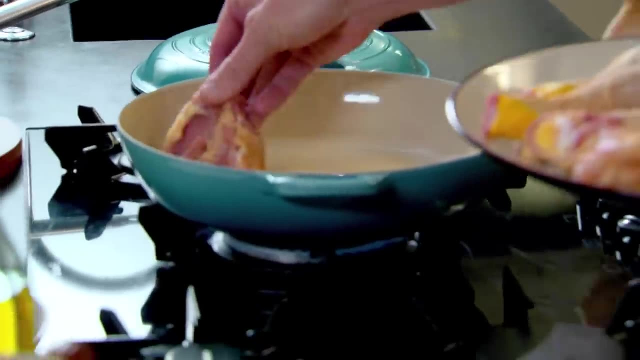 Put a tablespoon of olive oil in there. Couple of lugs, One, two. Good girl, Put the chicken in- Yeah, that's better- And you lay away. You get that nice and brown. You're getting good at this. 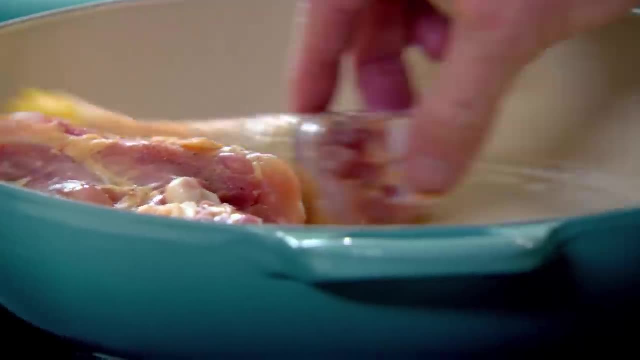 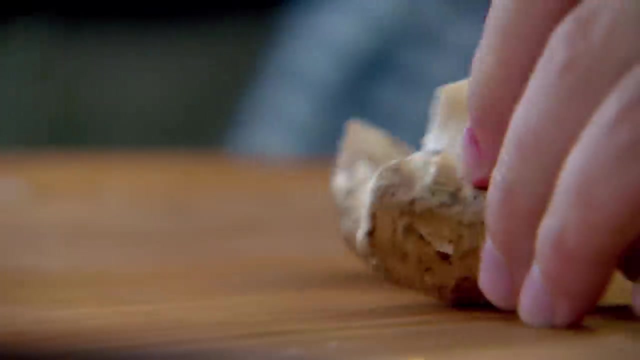 You are Skin side down, Yep, So we get the color on the skin. Now I just want you to cut the mushrooms in half, the belly, please. Thank you. OK, These are chestnut mushrooms. There are lots of different types of mushrooms, aren't there? 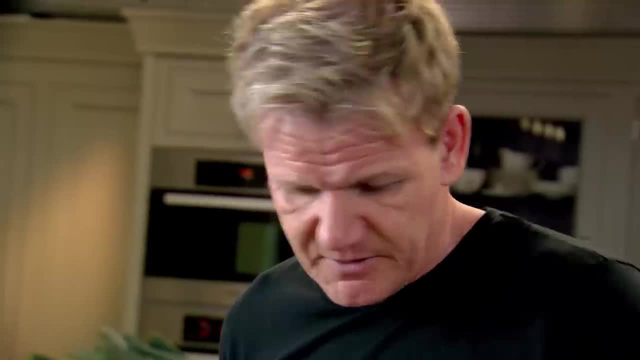 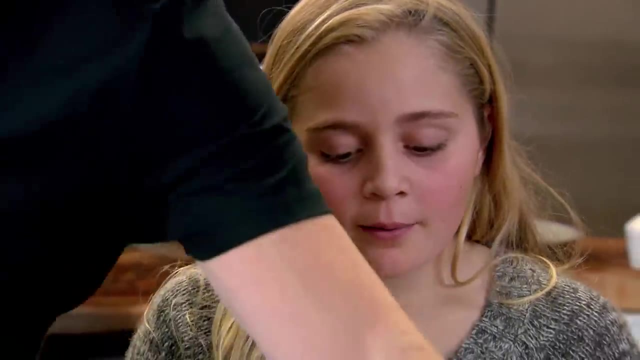 There are lots and lots of different types of mushrooms. Which one's your favorite? One of my favorites is the giroll mushroom. I like mushrooms that are a bit bigger than this And some dinners with mum. we cut out the middle, put pesto and cheese in it, and then we bake them. 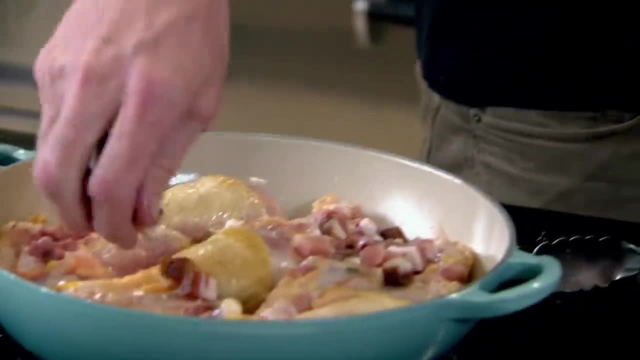 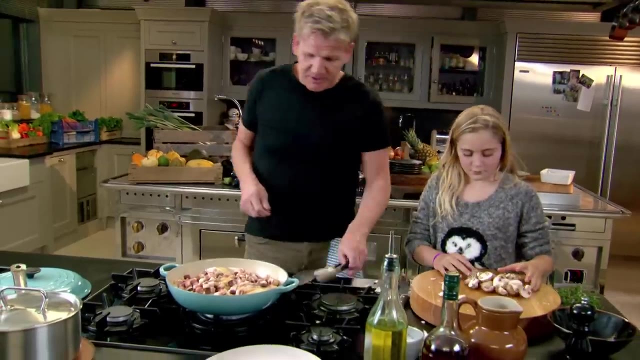 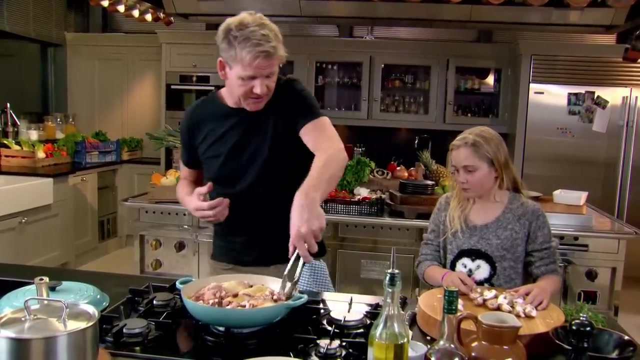 Oh, So I want you to sprinkle the pancetta over the chicken, please, Good girl, Nice, Put the mushrooms in, Not yet, because I'm going to get some color on the chicken first. OK, And as that pancetta starts to cook down, 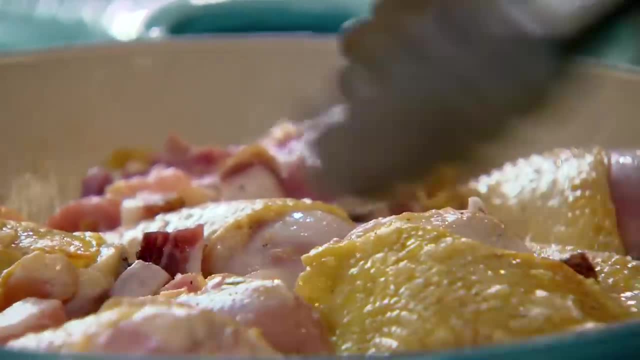 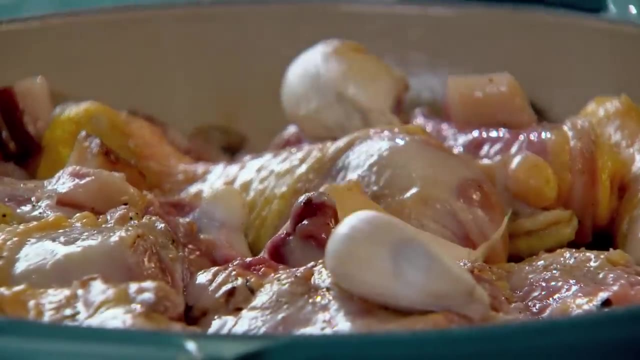 it puts a really nice flavor on the chicken. Yeah, So we're sort of sautéing everything. OK, Right, Garlic in, please, Good girl, Just throw them in, And I want you to sprinkle the mushrooms on top of that. 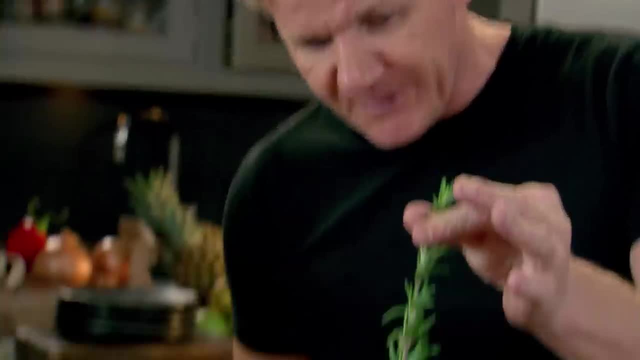 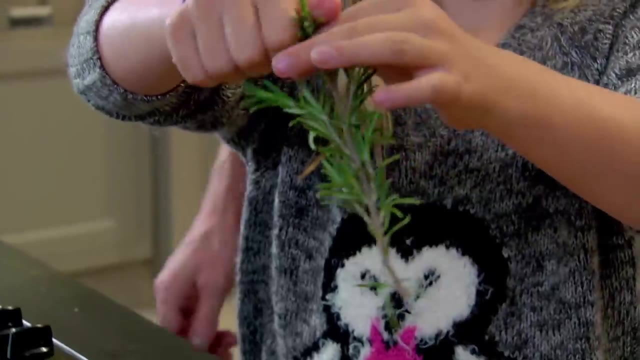 Good girl. And then there's the rosemary. OK, You get your fingers like that and you pull it down. You take it all off, Hold it, Put it down, Good girl. So now you've got the nice little rosemary sprigs. 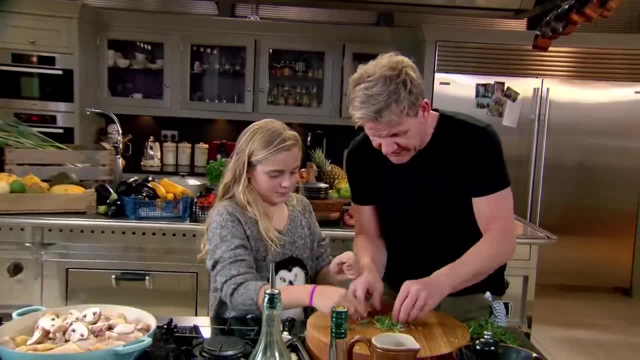 I want you to do the same with the thyme. Now the thyme flower is a little bit smaller. What different flavors do they give? So the thyme is a little bit sweeter, OK, And the rosemary is a little bit more savory. 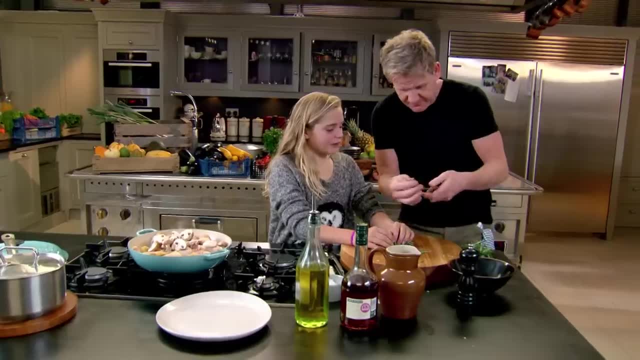 Which ones do you like? I like them both because they both give a nice flavor, Don't they? So bay leaf in. I'd like you to put that rosemary and thyme in there, OK, And then I'm going to add the garlic. 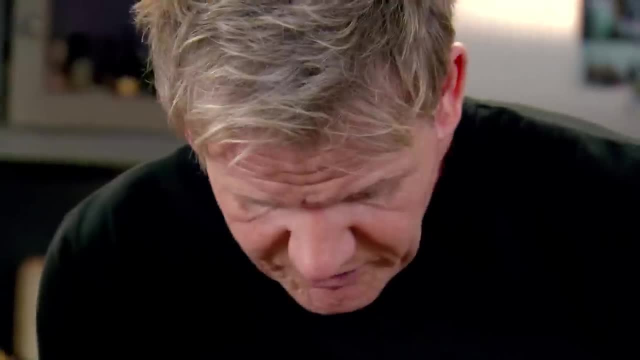 OK, And then I'm going to add the garlic, And then I'm going to add the garlic, And then I'm going to add the garlic, And then I'm going to add the thyme, And then I'm going to add the garlic. 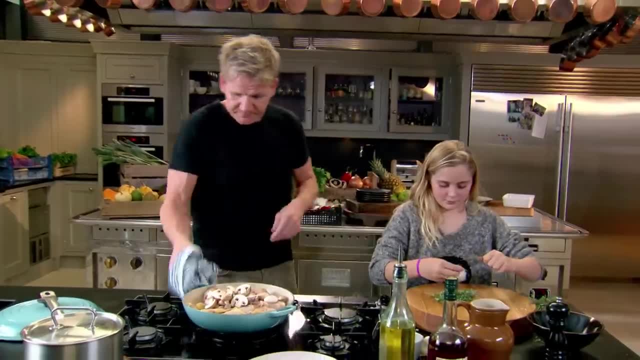 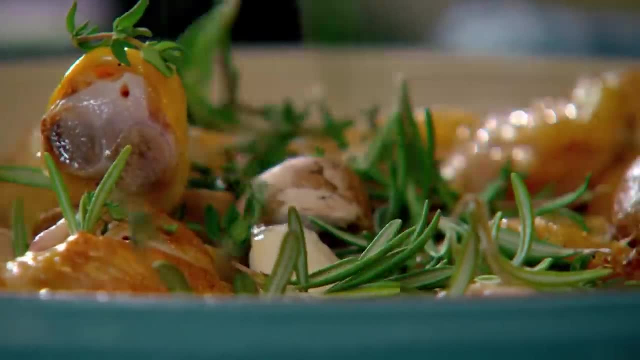 I like them both because they both give a nice flavor, Don't they? So bay leaf in. I'd like you to put that rosemary and thyme in there. please, Lovely Sprinkle it over, Right? I'd like you to stand back now, because we're going to flambe this. 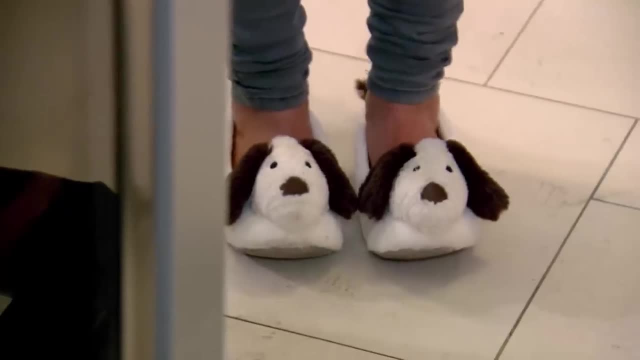 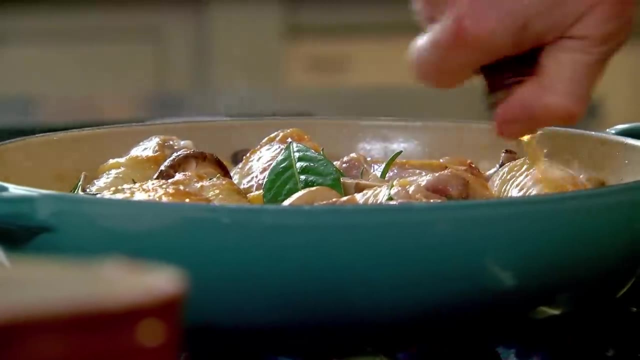 I do not want to get those little slippers caught on fire. What are the names? Rumpel and Judith. Judith, nice, OK, great, Ready, Yeah, In with the brandy. And then Judith: OK, Just tilt the pan, gently. 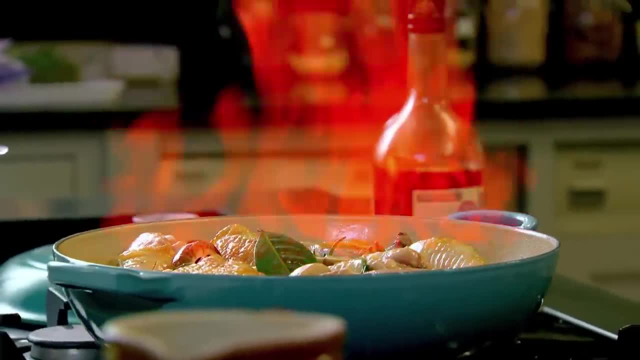 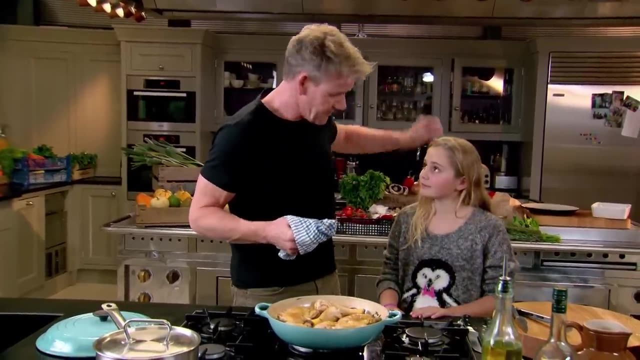 Whoa, Whoa. How cool is that? It's a bit magical, Beautiful, A bit like a cauldron. All the cognac has been flambeed, so there's no raw alcohol anywhere, So we've got a really nice, deep, rich flavor. 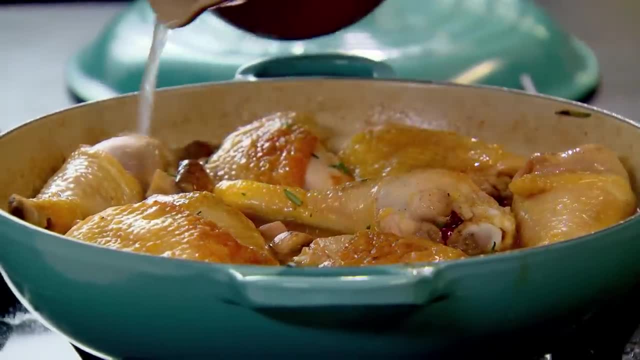 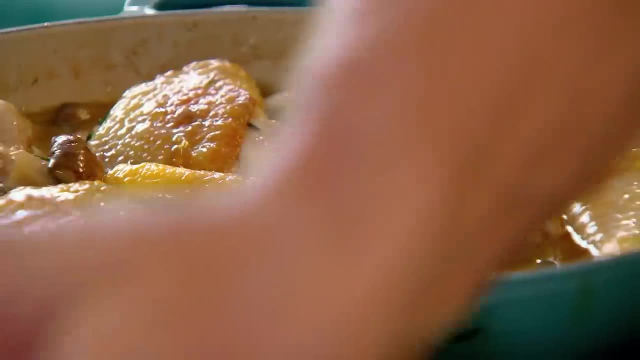 I'm going to add my chicken stock. You know, Rumpel likes that, Not my slipper, Rumpel. Rumpel the dog. Ah, Rumpel the dog, Well, he likes chicken stock. Yes, When he's a good boy, he gets it with his biscuits. 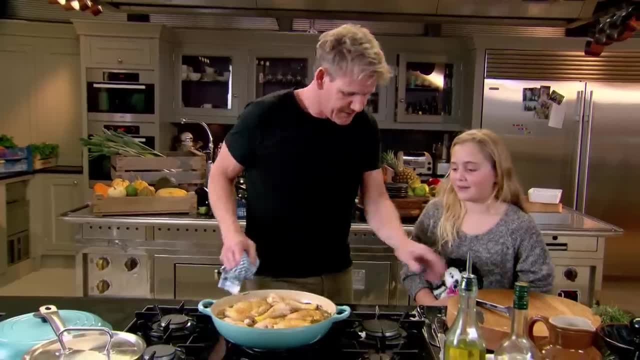 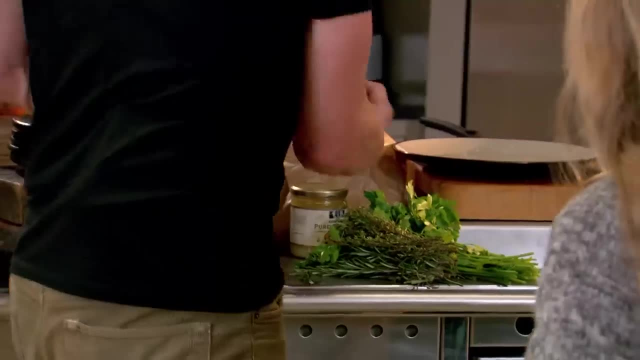 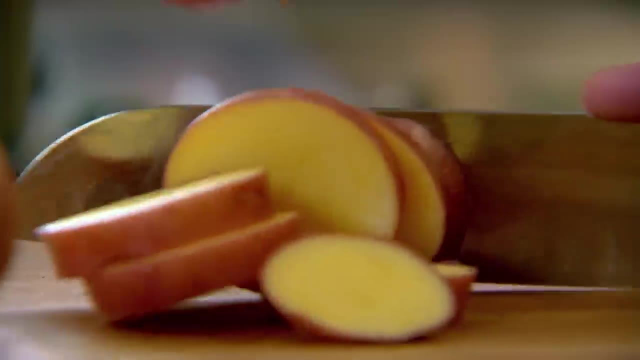 OK, It's gone in like wow, really quickly. Simmer and reduce the stock for around ten minutes. Now we're going to cook the most amazing potatoes. Sautéed potatoes are really simple to make and absolutely delicious. Start by slicing the potatoes into finger-width pieces. 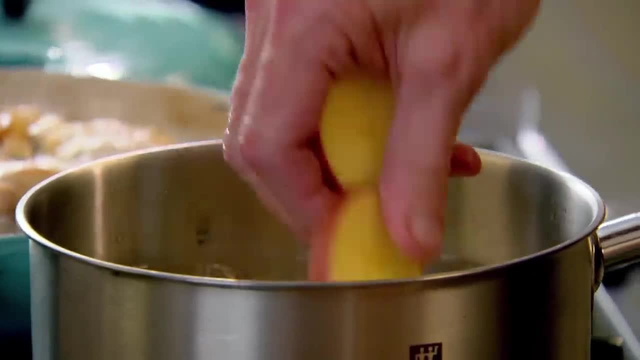 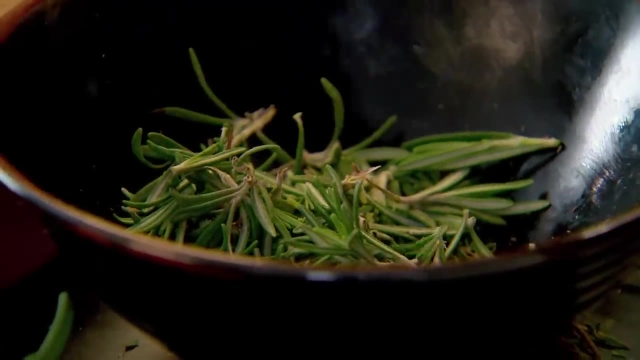 Then parboil them for five to six minutes. When you cook something like rosemary or thyme or basil, does it slowly let off the flavor into the pot, or Very much so. In a hot pan add a tablespoon of goose fat. 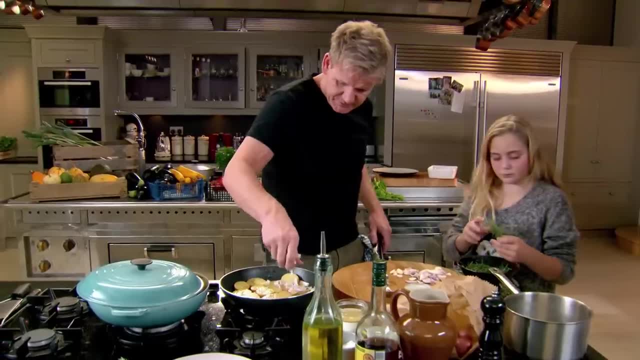 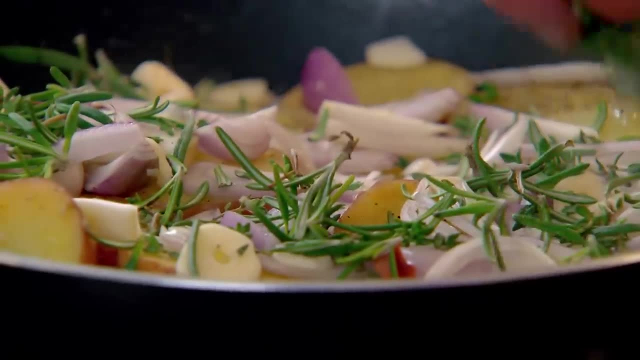 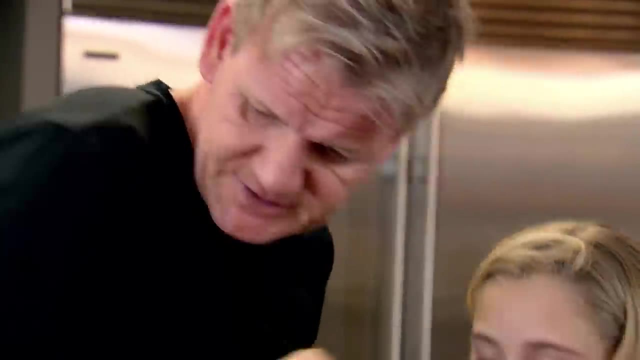 and sauté the potatoes until they turn golden And add in shallots, garlic, rosemary and thyme. That goes in Over the top And that goose fat now is starting to fry the potatoes. You just leave that sat there. 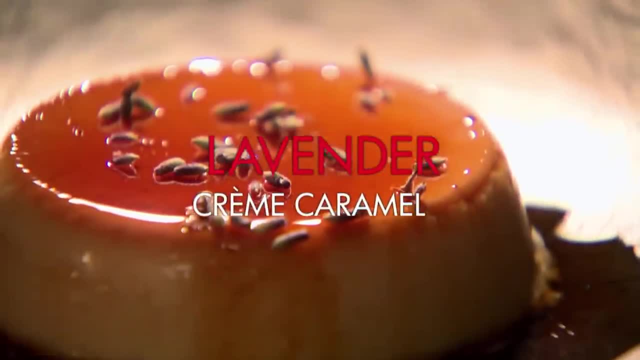 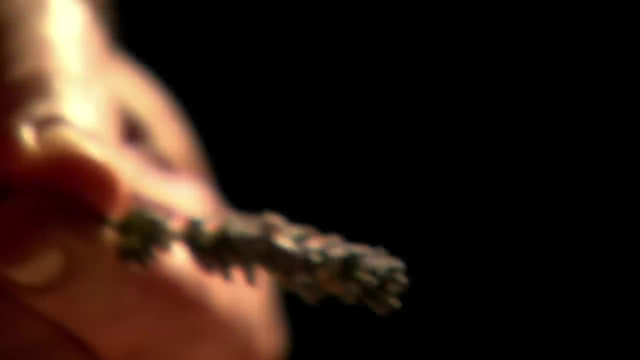 To complete my ultimate French dinner, my version of a classic: a glorious lavender creme caramel for dessert. The first job is the lavender sugar. You can buy this ready-made or simply add dried edible sprigs of lavender to caster sugar and store. 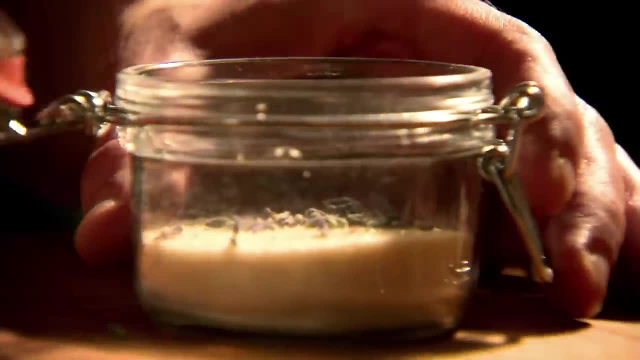 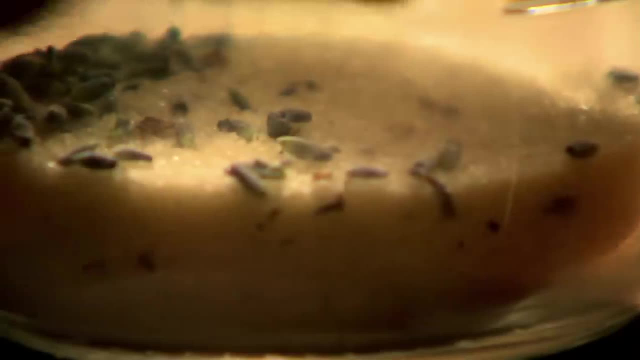 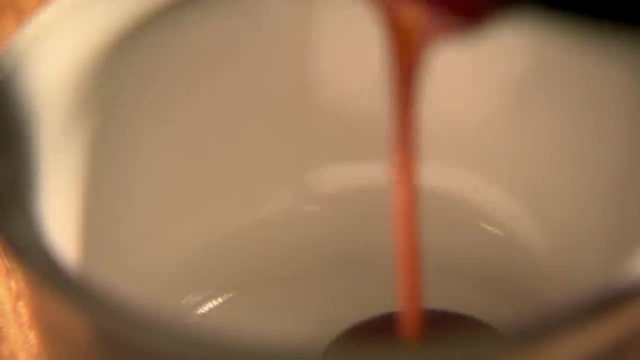 You can also try this trick with vanilla pods and cinnamon to bring new subtle flavors to sweets and baking. For the creme caramel: melt plain caster sugar until it turns dark golden, Pour into ramekins, sprinkle with lavender flowers and cool Now to make a simple custard.